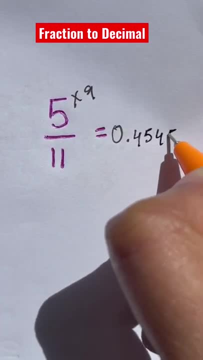 45, so you just keep writing 4, 5,, 4, 5 and so on. So that's just 0.45 recurring. 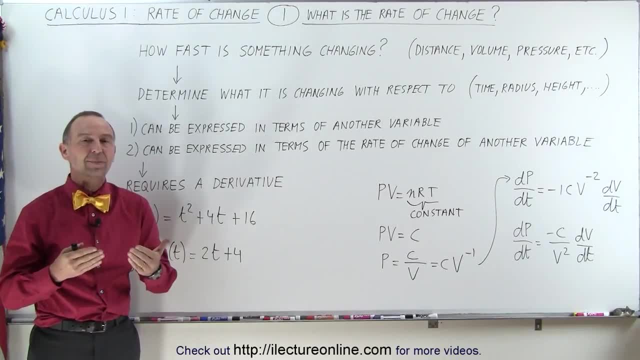 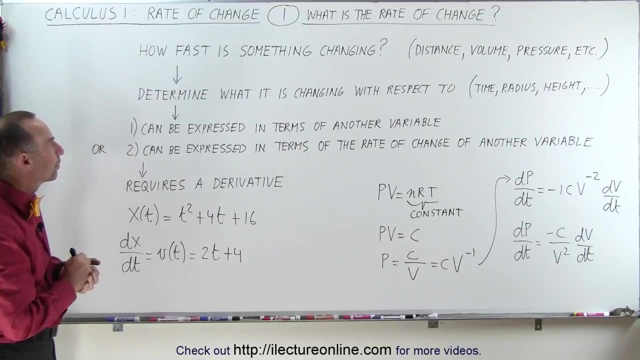 Welcome to our lecture online. Now let's take a look at another concept in calculus called the rate of change. What is it? What's the definition of the rate of change? Well, the rate of change indicates how fast something is changing. Now, that could be the distance, the volume. 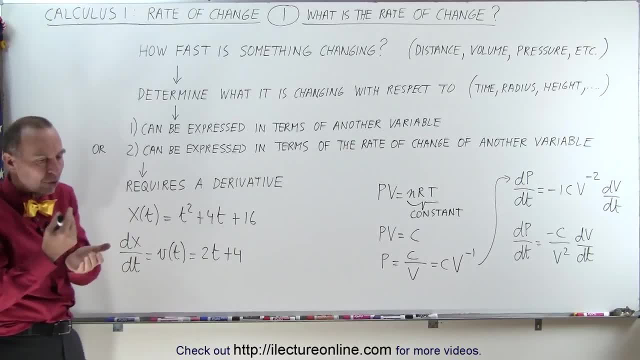 the pressure of something. it could be any number of things. So you're asking the question: how fast is something changing? That's what we mean by the rate of change. It determines what is changing with respect to something else, That something else could be time. 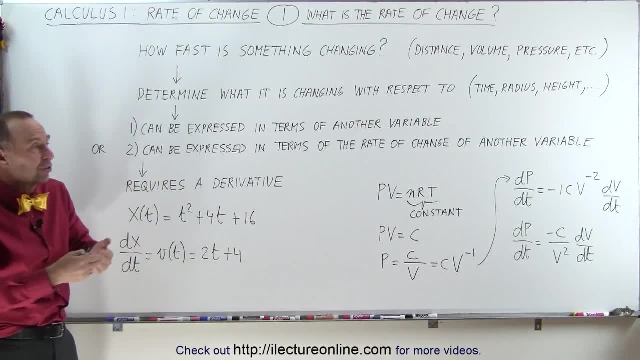 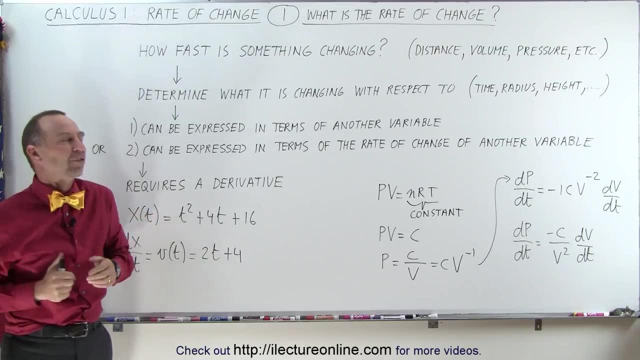 radius, height and so forth. So how fast is the volume changing as a function of the radius, for example? So that's where we always look for something is changing with respect to something else, And it can be expressed in two ways. We can express it in terms of another variable. 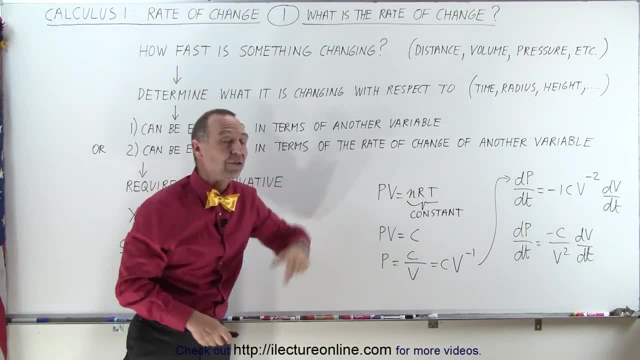 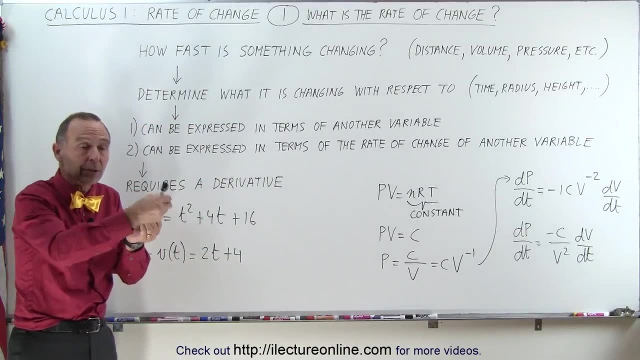 or it can be expressed in terms of the rate of change of another variable, or a combination thereof. So So, when we're looking at how fast something is changing, it could depend on another variable, it could depend on the rate of change of the other variable, or it could depend on a combination. 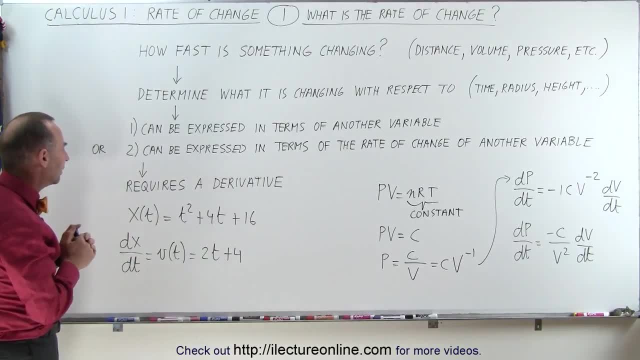 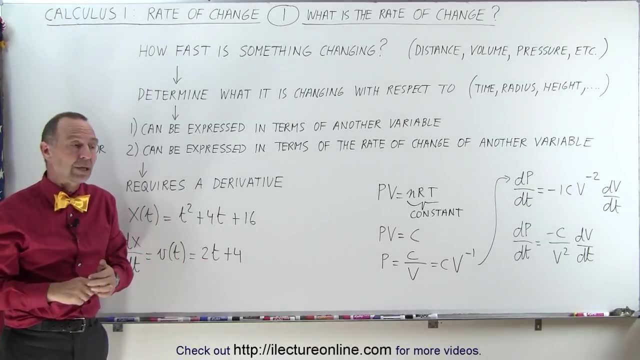 of the two. So what does that mean? Well, first of all, it requires a derivative. A derivative, by definition, is the rate of change of something, or how fast something changes relative to something else, or how much something changes relative to something. 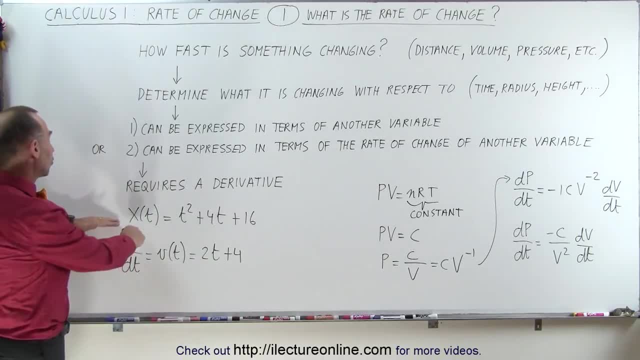 else. So if we take, for example, an equation that describes the position of something with respect to time, and here we can see, that's equal to t squared plus 4t plus 16.. If we want to know how fast something is changing with respect to time, in this case how fast.